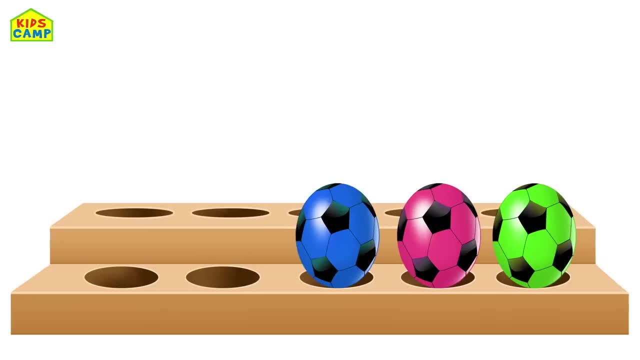 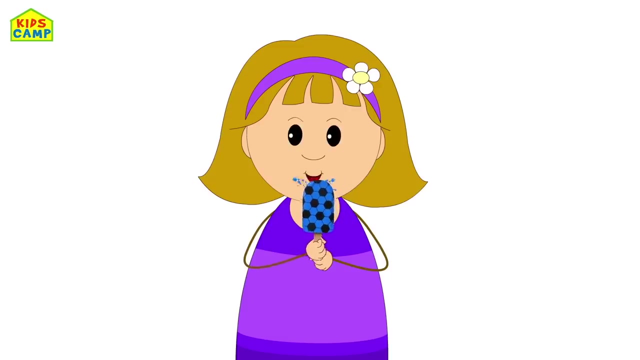 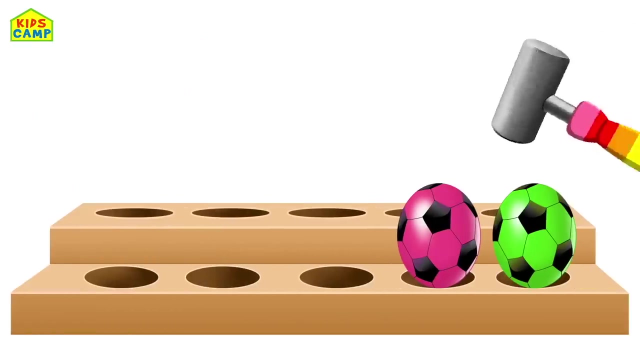 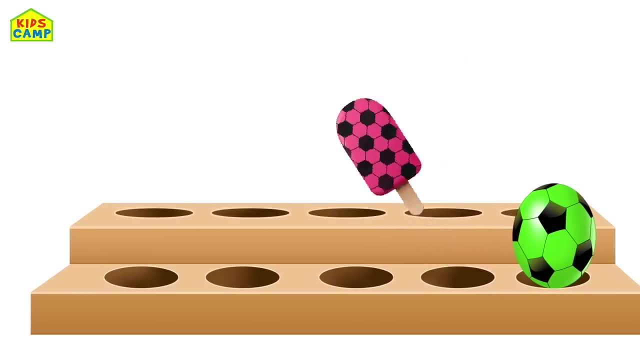 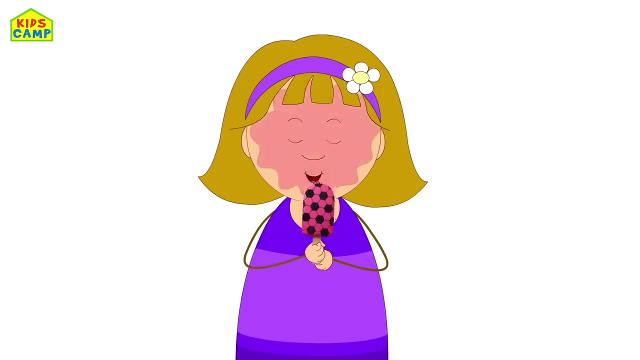 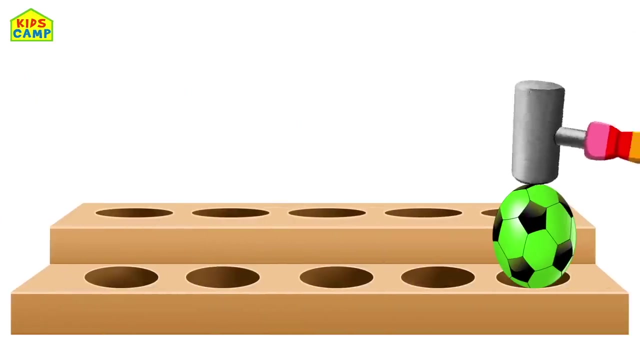 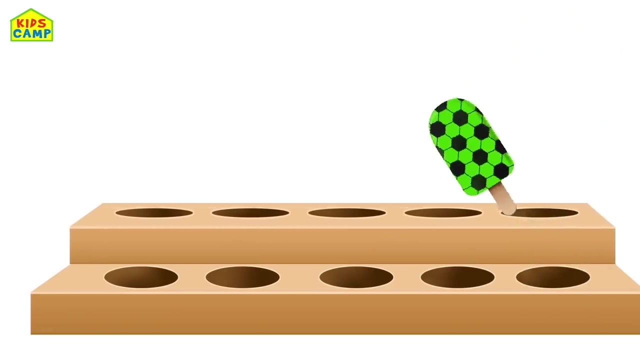 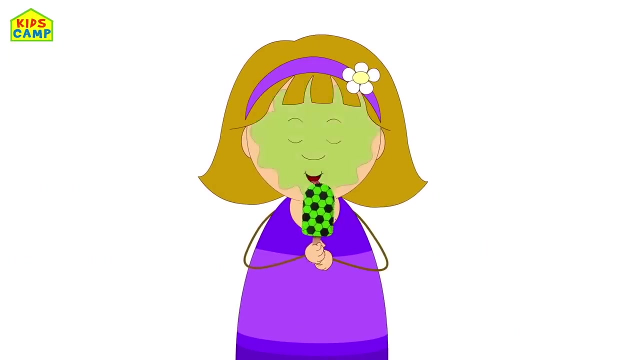 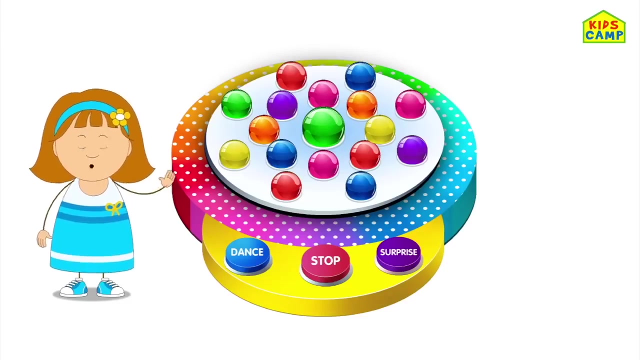 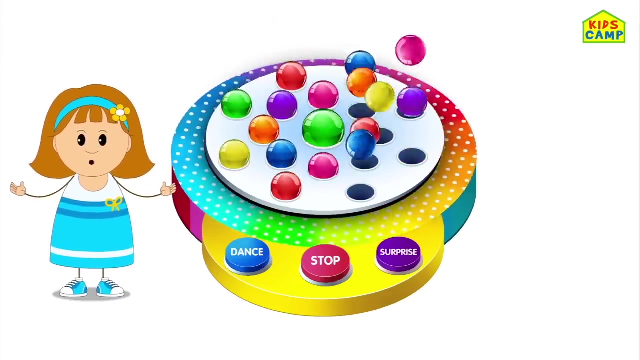 Yellow, Blue, Blue, Blue, Blue, Blue, Blue, Pink, Blue, Blue, Blue. Hi, I am Elly. today we are going to spin the dancing wheel of surprises. Ready, Let's spin the wheel. Surprise wheel goes round and round, round and round, round and round. 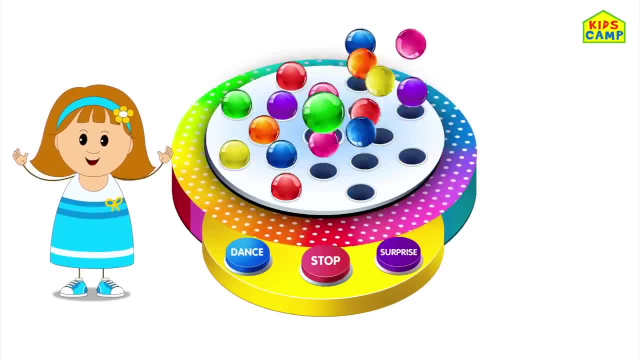 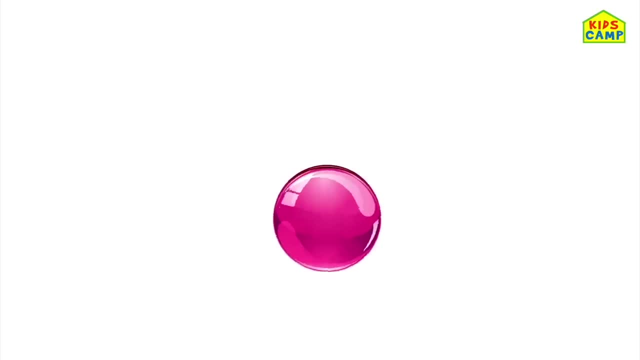 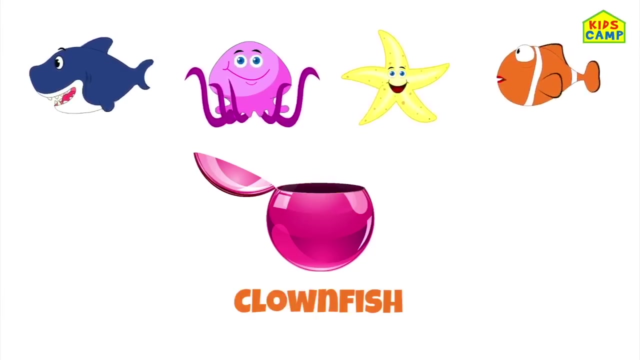 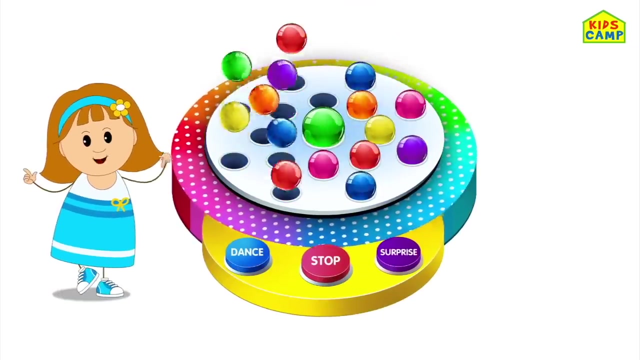 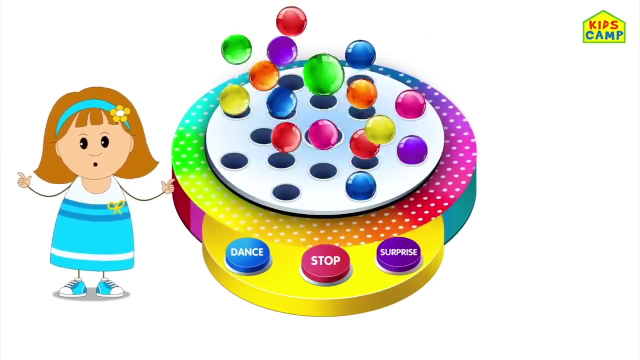 Surprise wheel goes round and round all day long. Wow, Surprise Shark, Blue, Jellyfish, Pink, Starfish, Yellow, Clownfish, Orange- Let's spin the wheel again. Surprise wheel goes round and round, round and round, round and round. Surprise wheel goes round and round all day long. 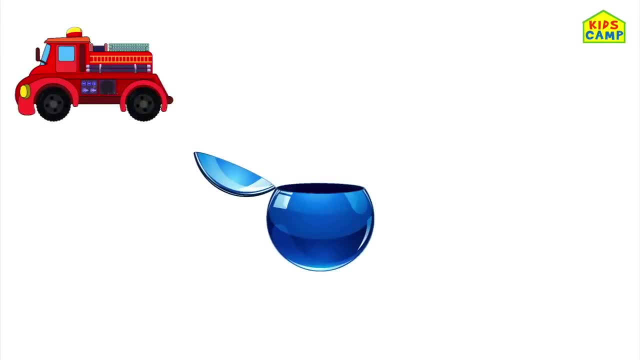 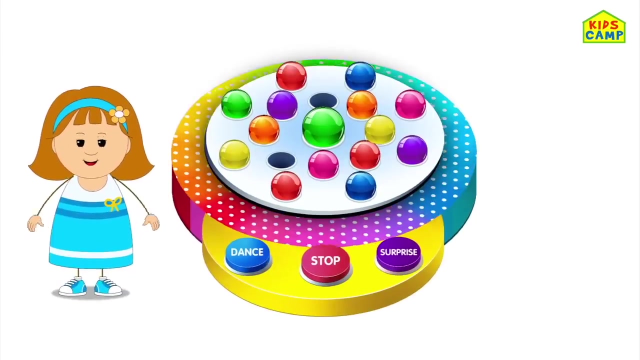 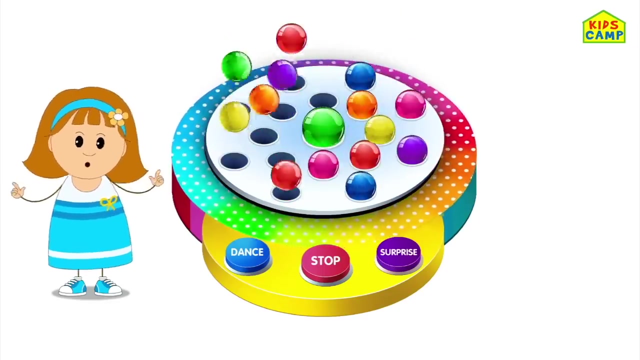 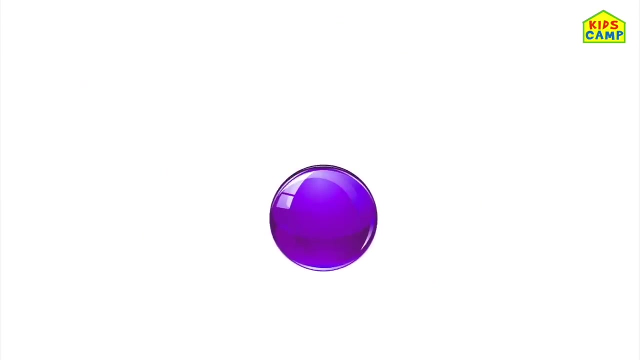 Yay Surprise. Fire truck- Red Helicopter, Blue, Ice cream truck, Pink, Car- Yellow. What will the next surprise be? Yummy fruit, yummy fruit. where are you Here? I am, here, I am. how do you do? Yay, Surprise. 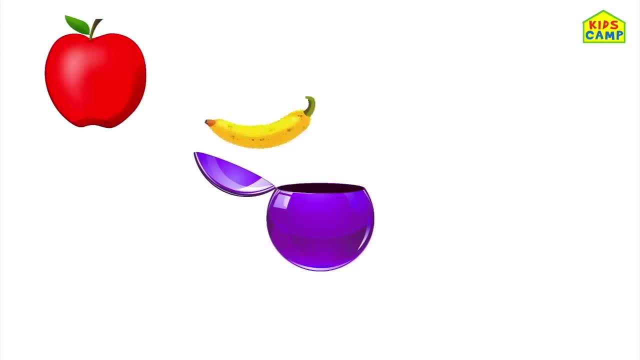 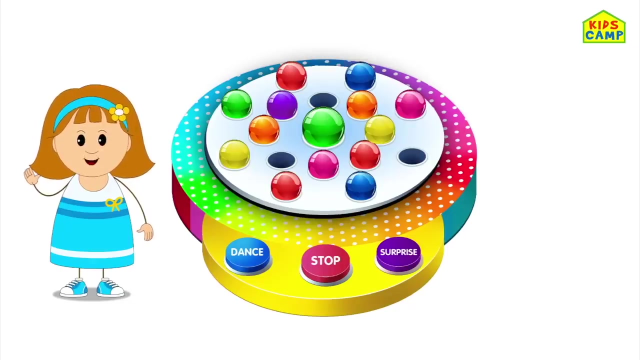 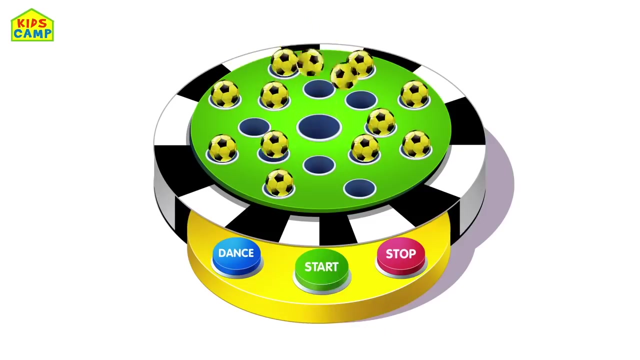 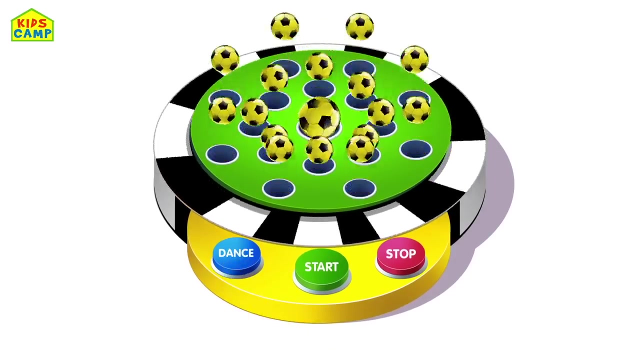 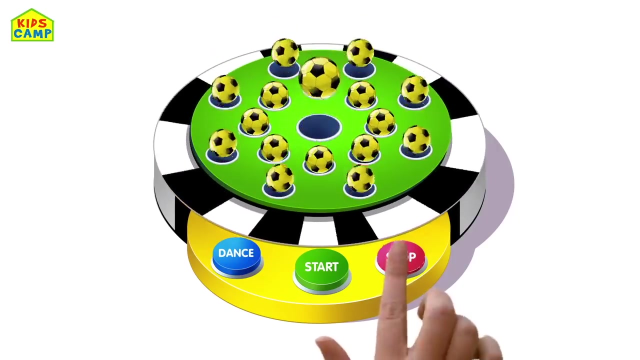 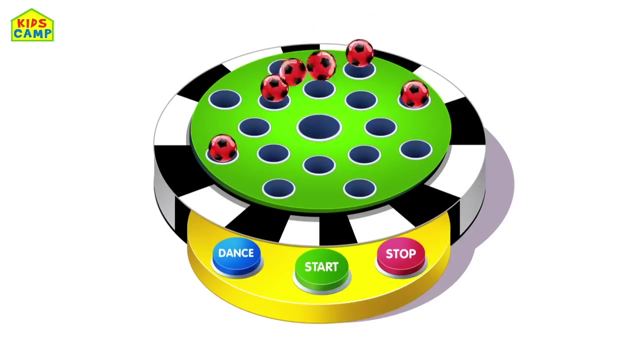 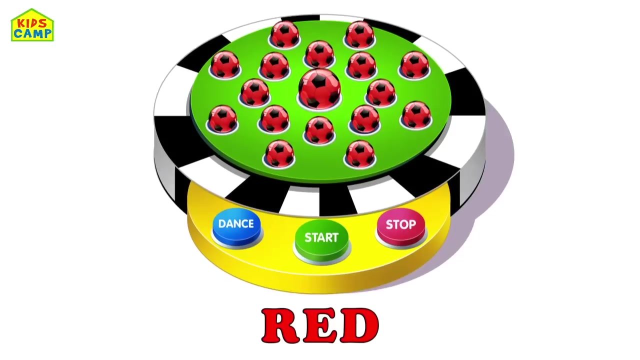 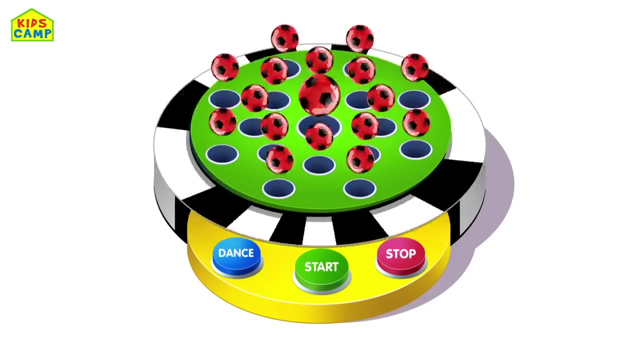 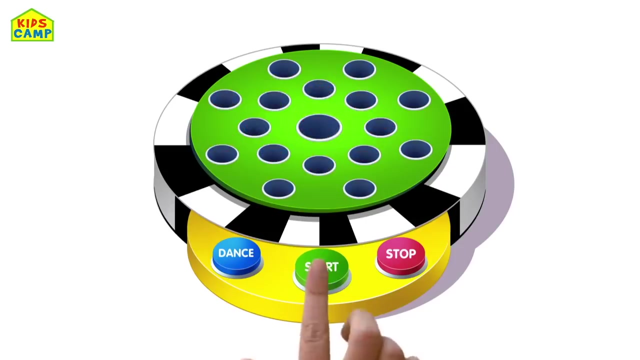 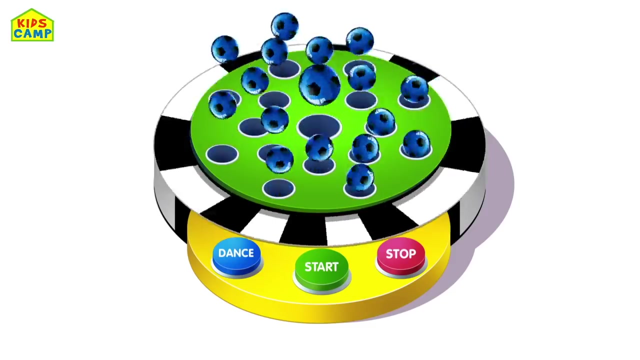 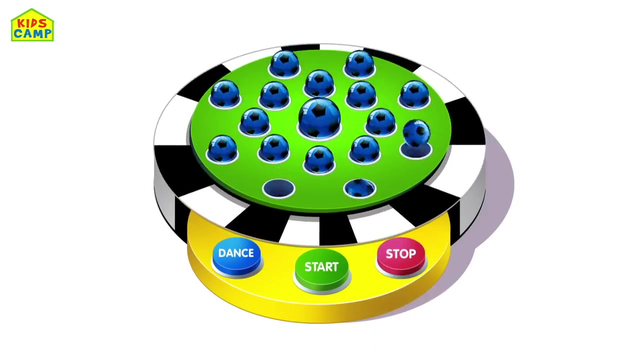 Apple, red banana, yellow, orange, orange bear, green, Yay, This was so much fun. Bye-bye, Yellow Yay. Red Yay, Blue Blue Yay, Blue Blue Orange. 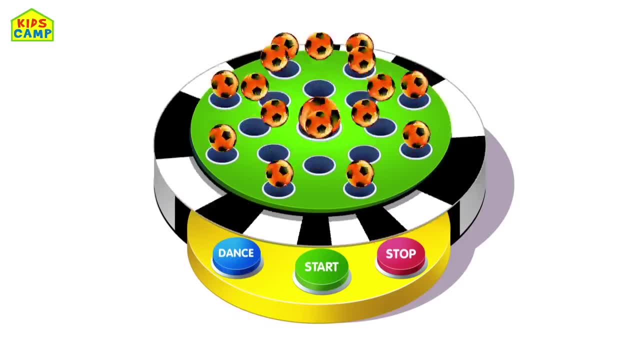 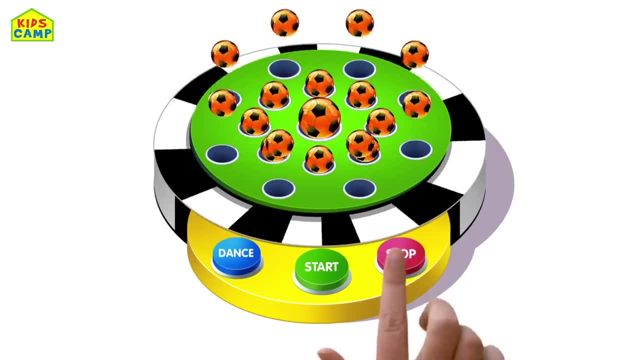 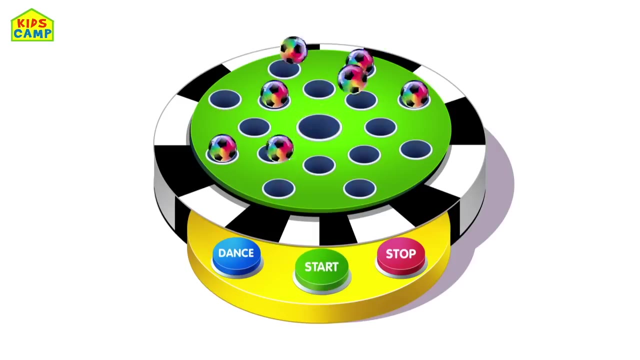 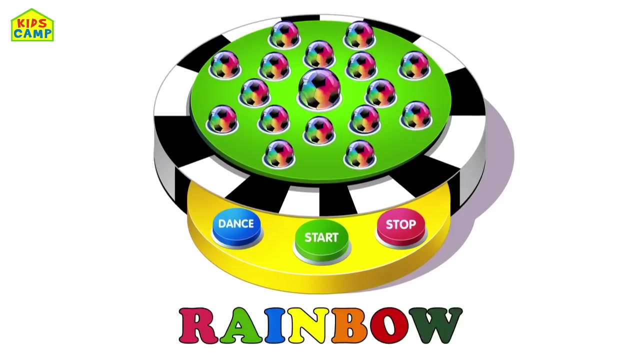 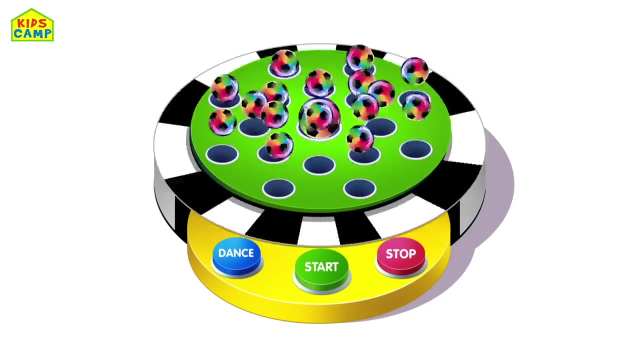 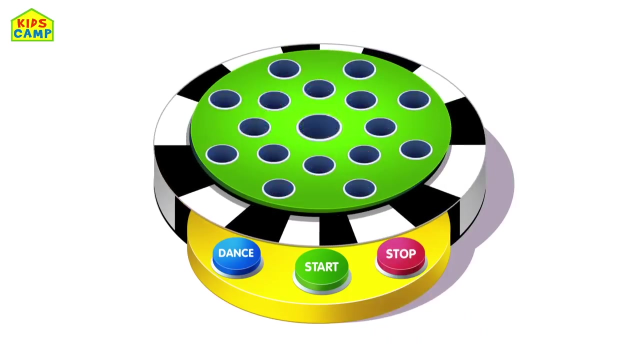 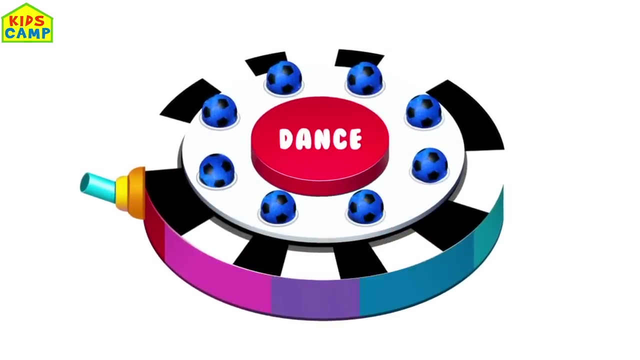 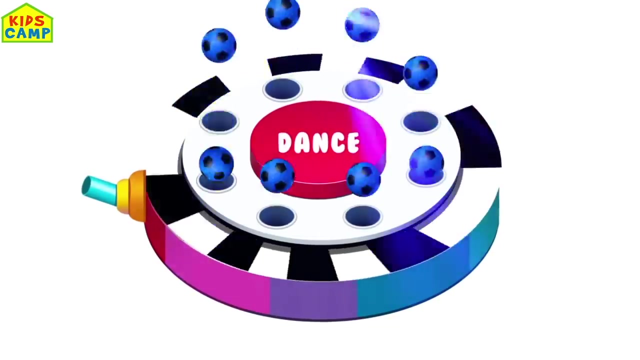 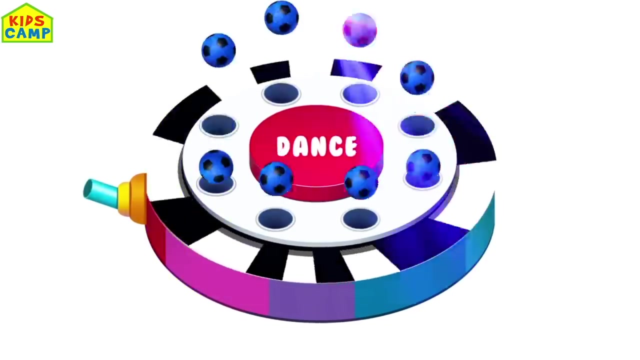 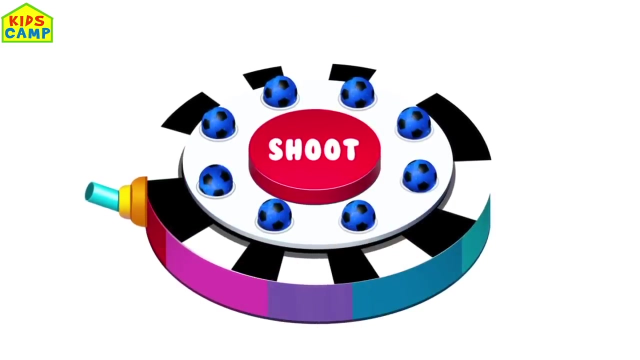 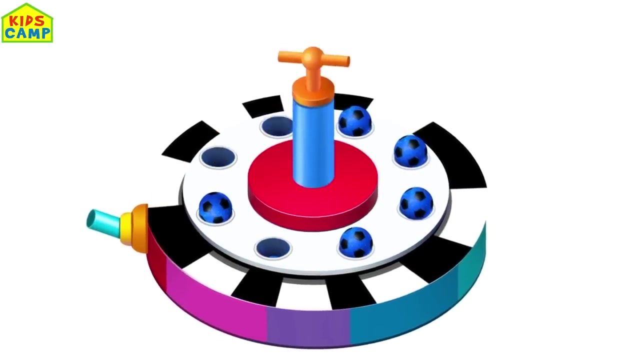 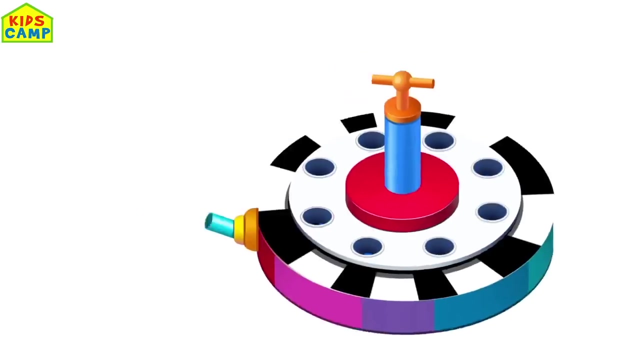 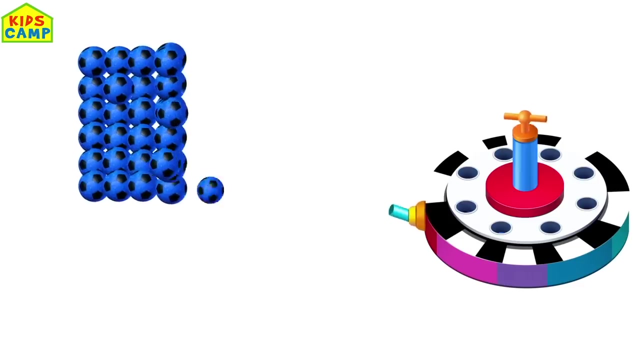 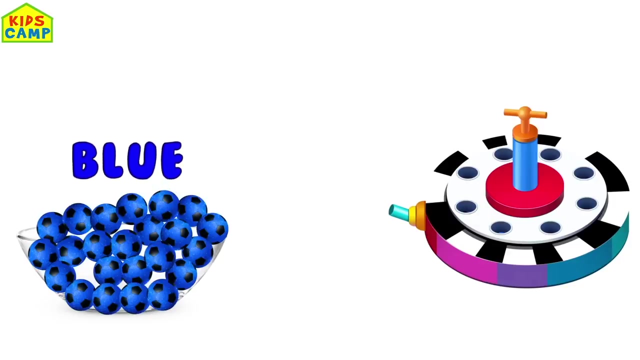 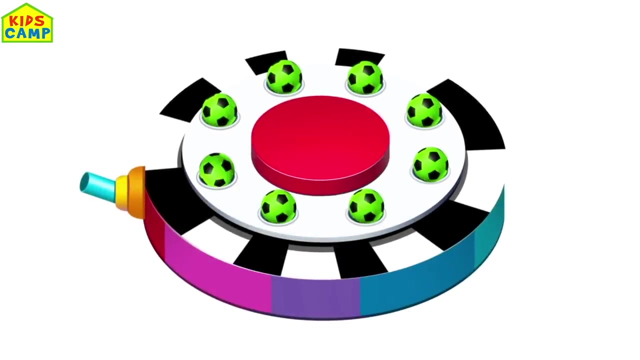 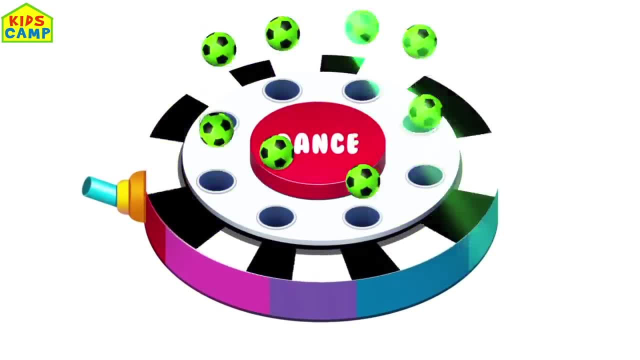 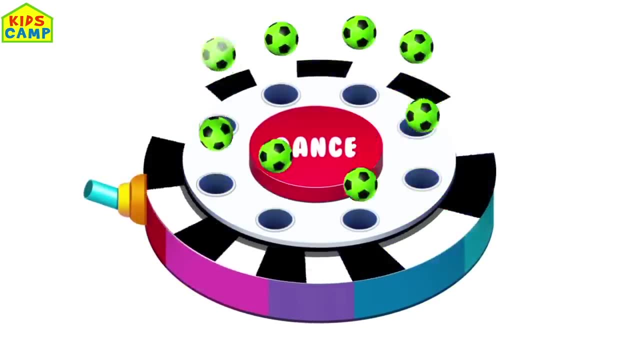 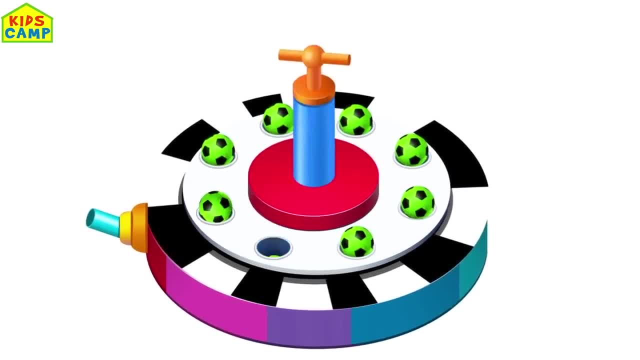 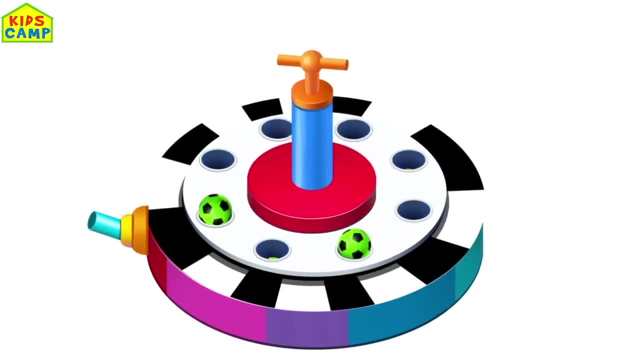 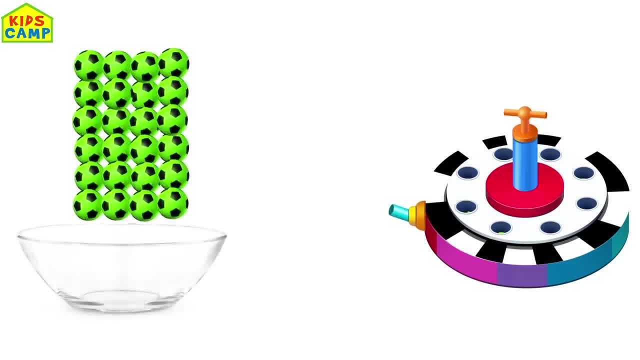 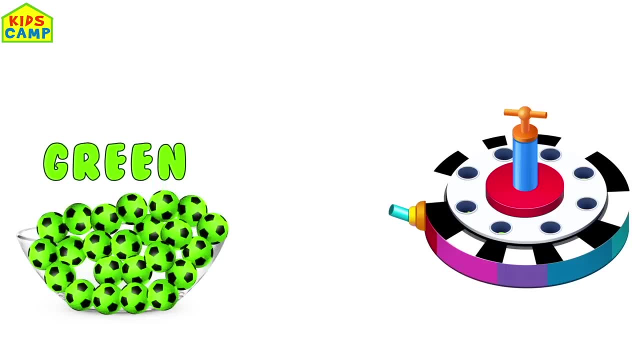 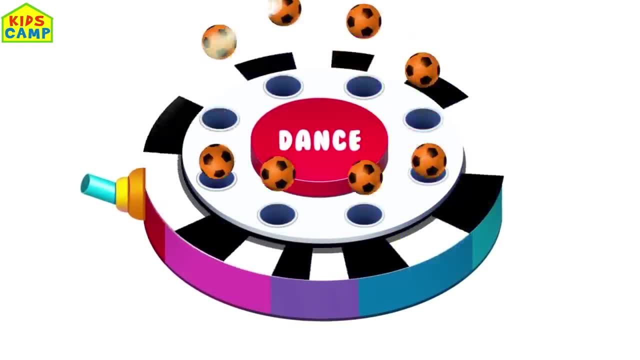 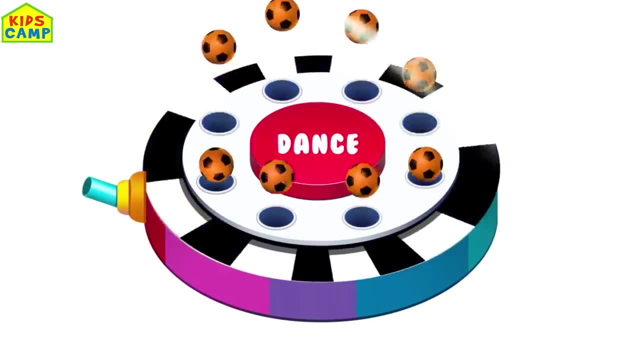 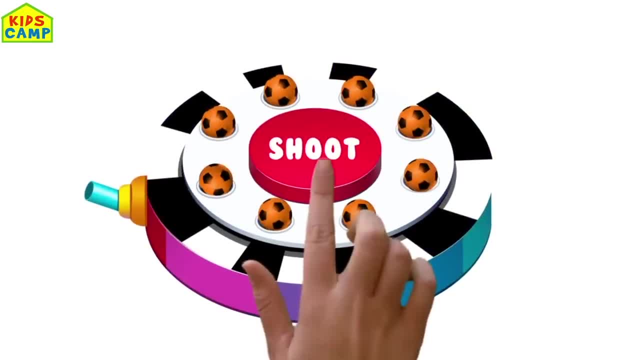 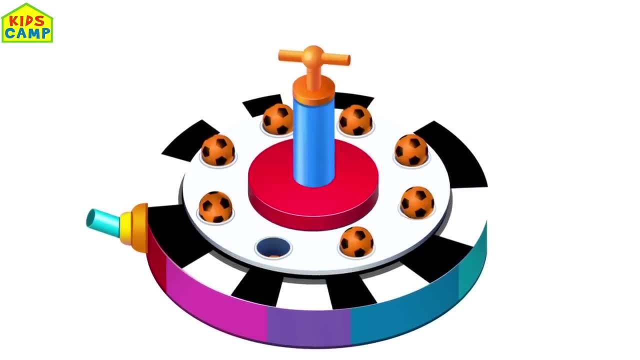 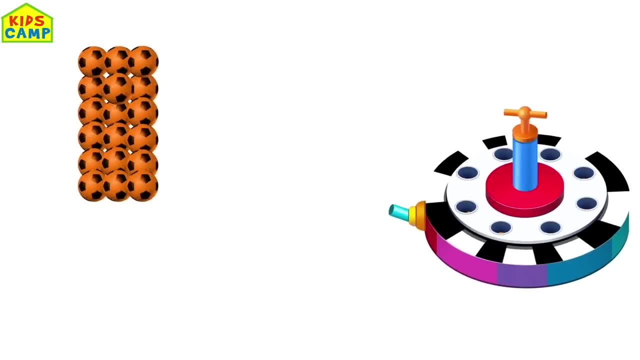 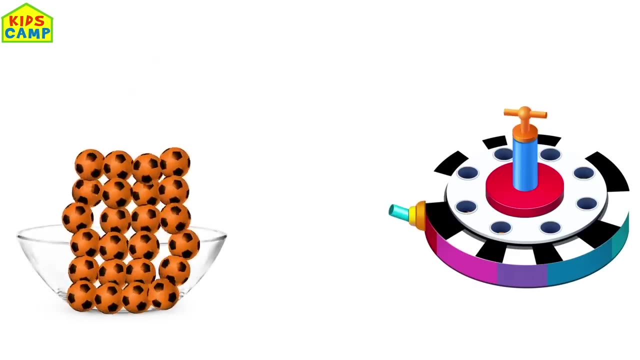 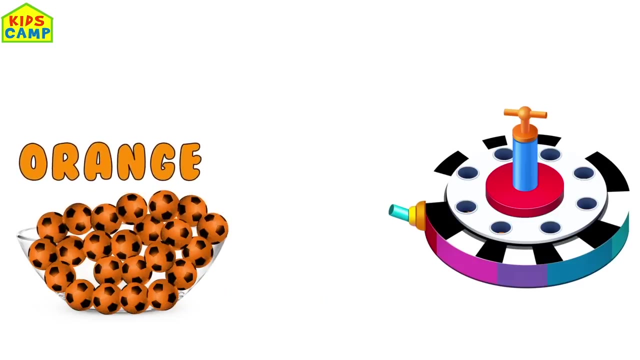 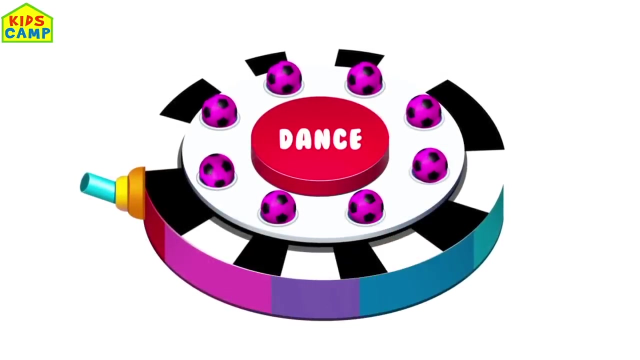 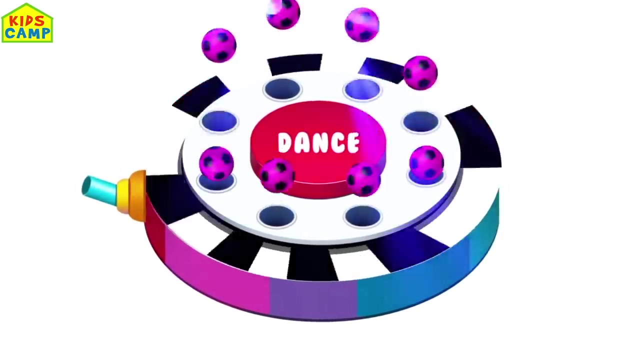 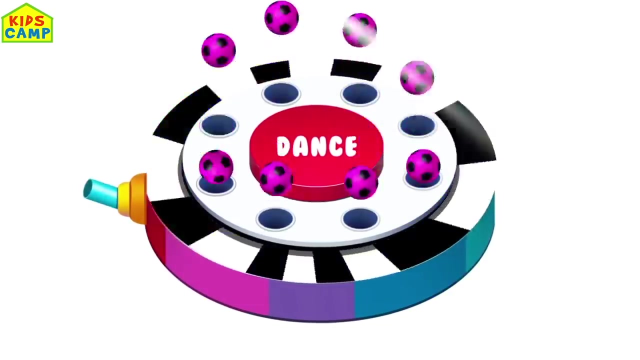 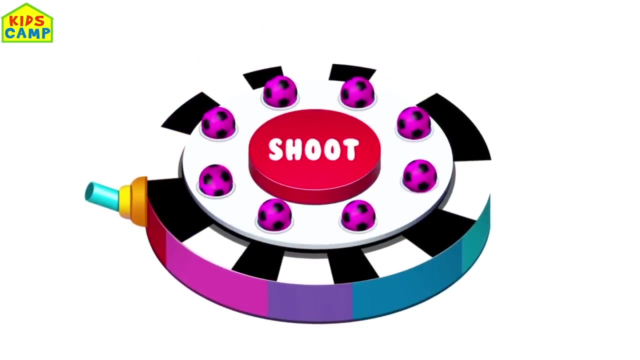 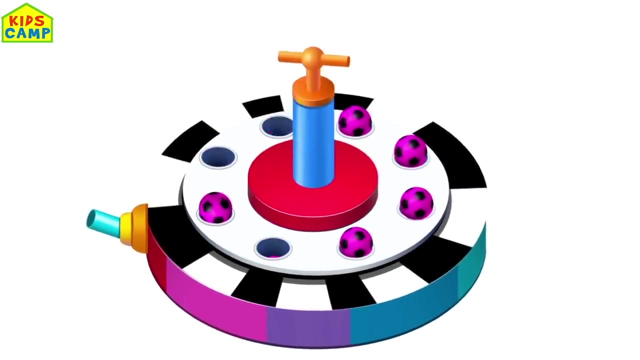 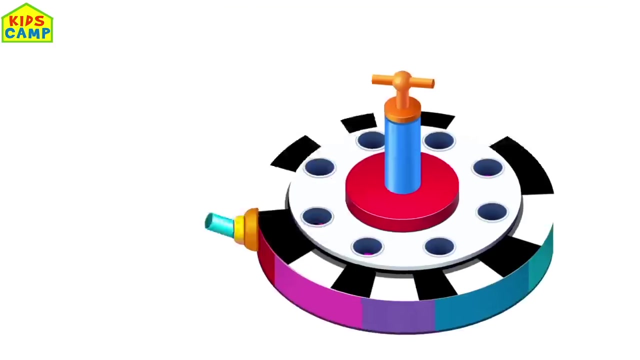 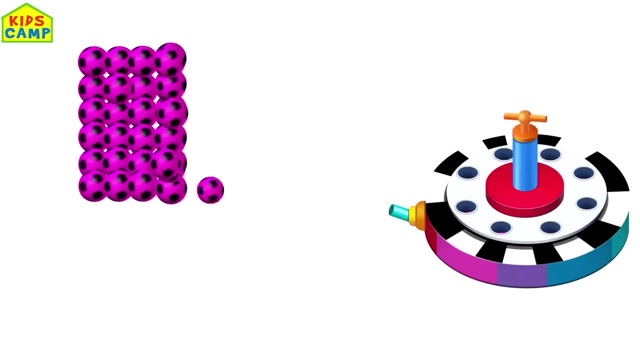 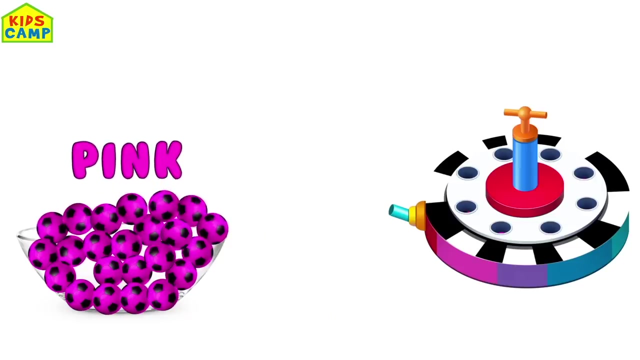 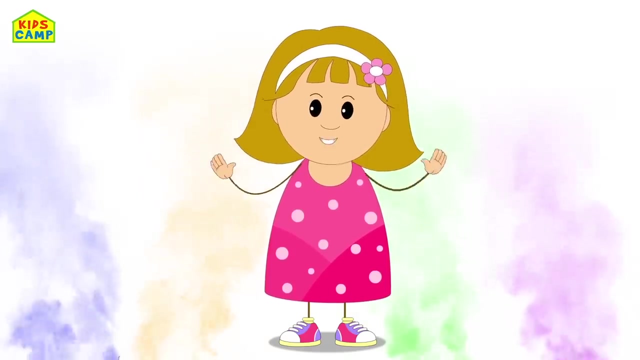 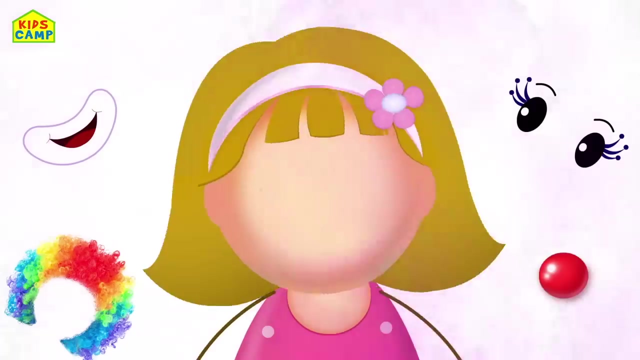 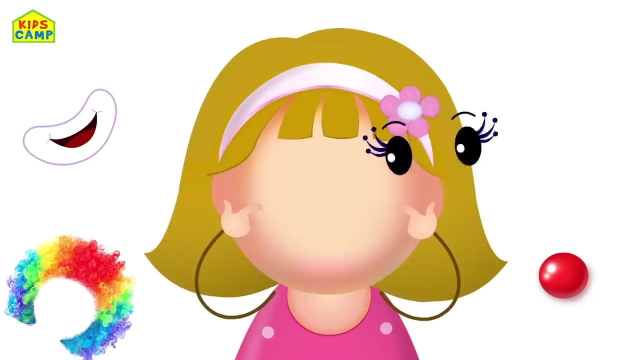 Game on Bingo Orange. Oh yeah, Game on Bingo Pink. Hi, I'm Ellie, Let's get a little funny today. Here we go, Here we go. Funny eyes, funny eyes. Where are you Here? I am, here, I am. 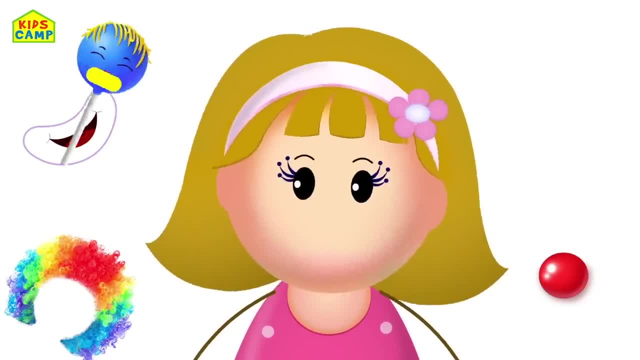 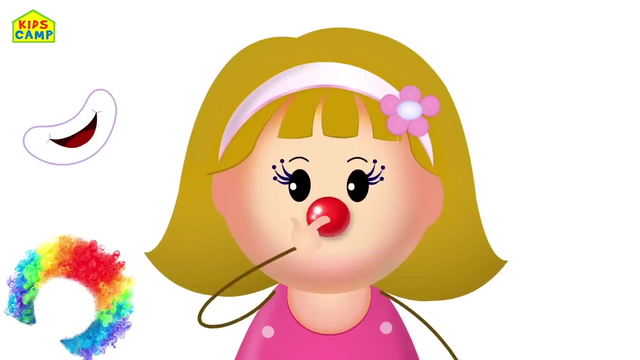 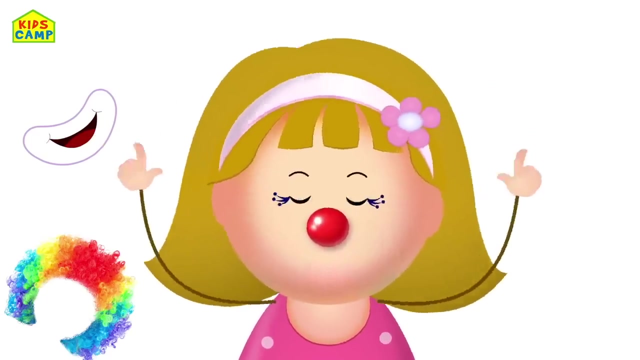 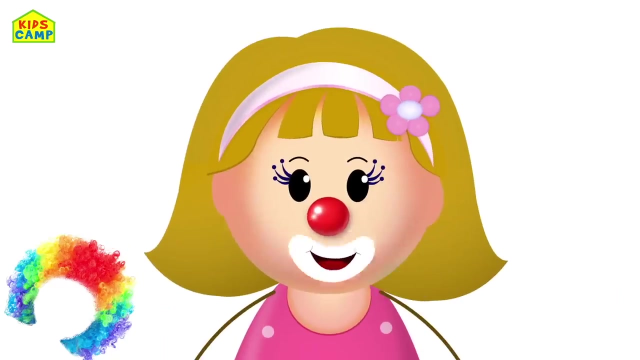 How do you do Funny nose? funny nose. Where are you Here? I am here, I am. How do you do Funny mouth, funny mouth. Where are you Here? I am, here, I am. How do you do? I already look funny. 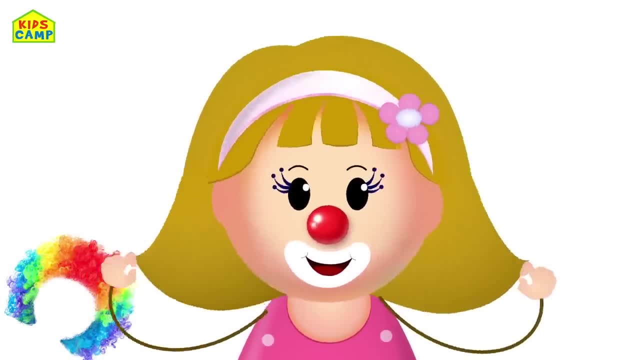 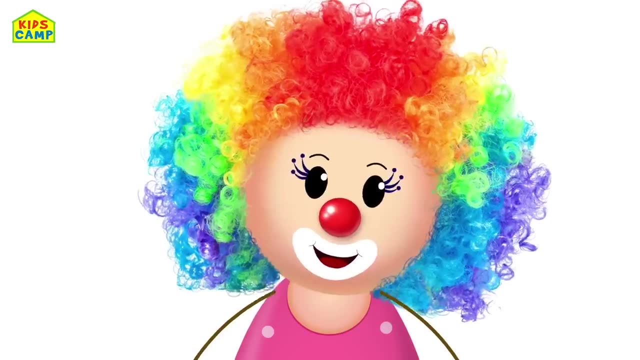 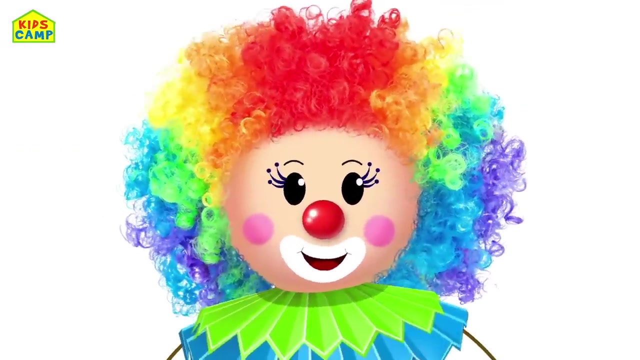 Funny hair, funny hair. Where are you Here? I am, here I am. How do you do So colorful Funny clown, funny clown. Where are you? That's me Here, I am, here I am. How do you do? I am so funny. 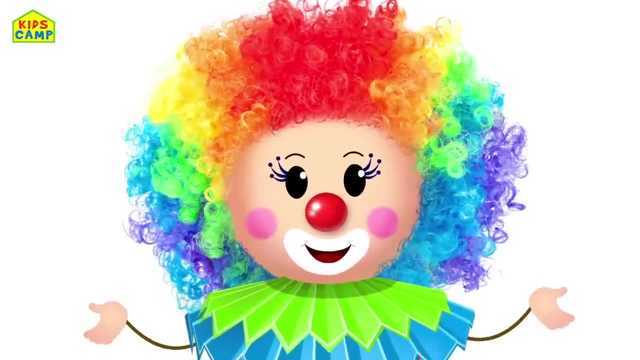 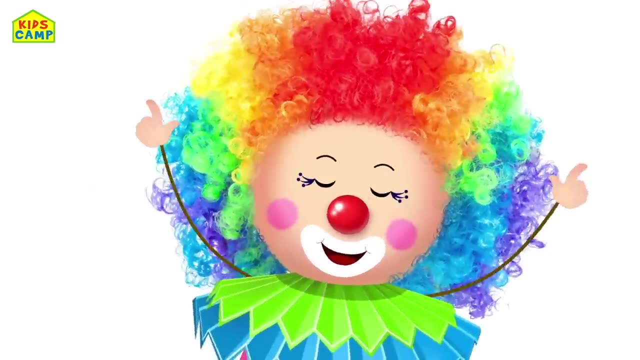 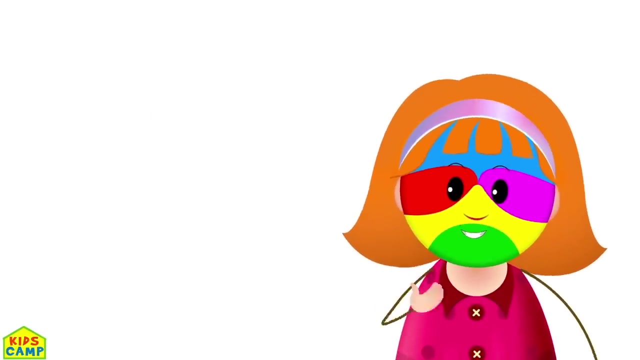 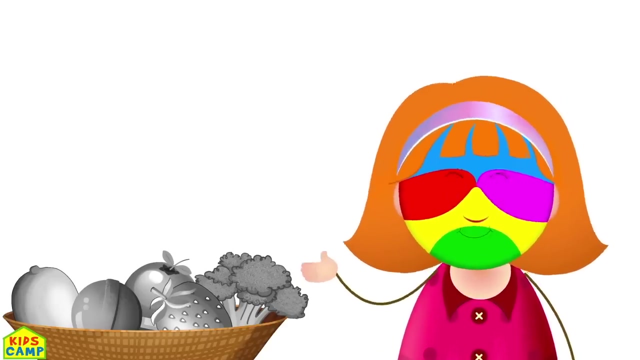 Bye-bye. Hi, I'm Ellie. Look at my face. It's all painted. I have a basket full of surprises for you and they need to be colored. Will you help me? I have a basket full of surprises for you and they need to be colored. 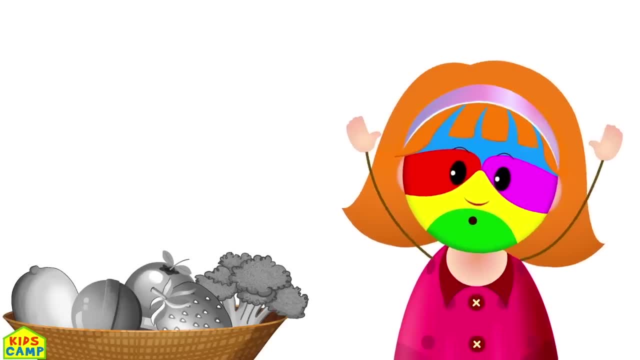 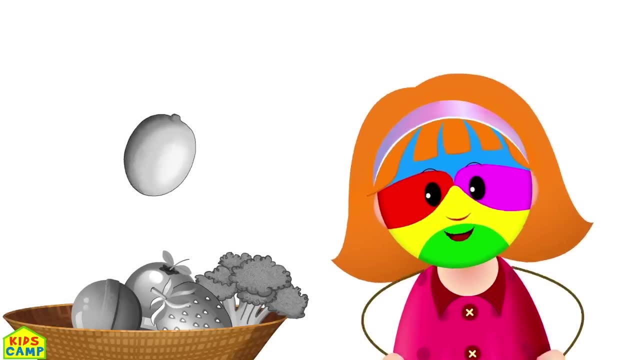 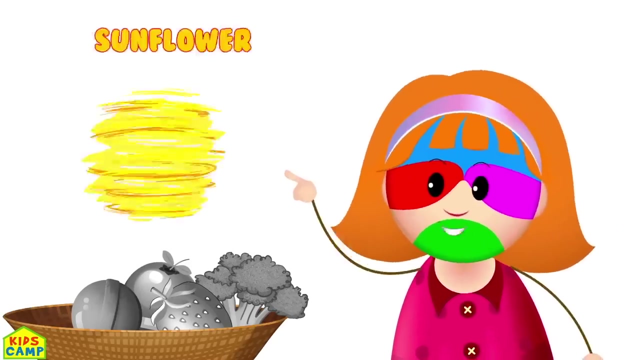 Will you help me? Yes, Thank you, Here we go. What color is the lemon? What color is the lemon? Yellow, yellow. the lemon is yellow Like the star, like the sun, like the sunflower. This is so much fun. 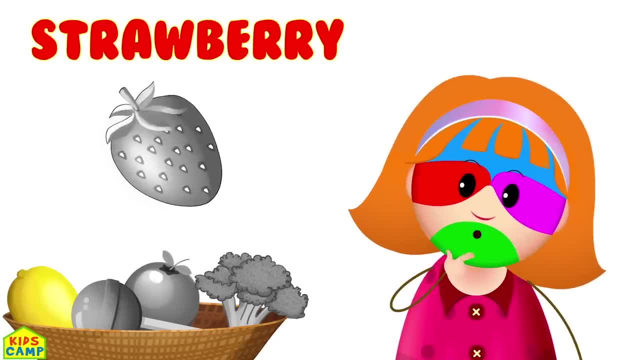 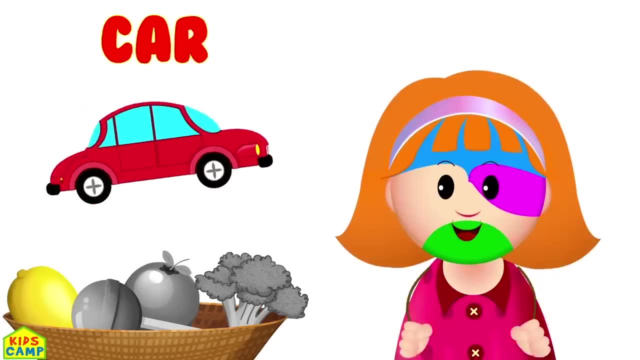 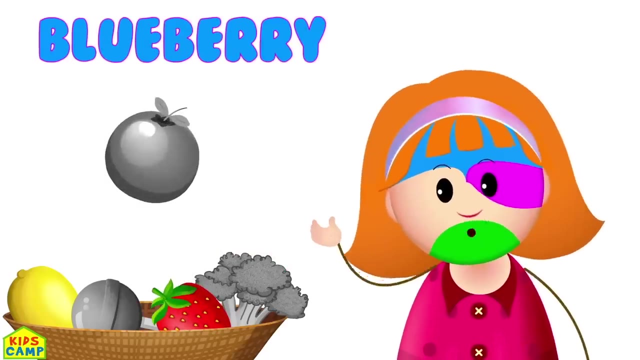 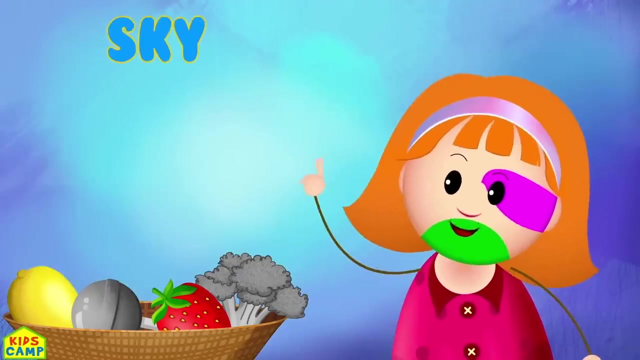 What color is the strawberry? What color is the strawberry? Red, red- the strawberry is red Like an apple. like an apple, Like a car. You're doing great, Like a superstar. What color is the blueberry? What color is the blueberry? Blue, blue- The blueberry is blue Like the sky, Like a cloud. This is fun. 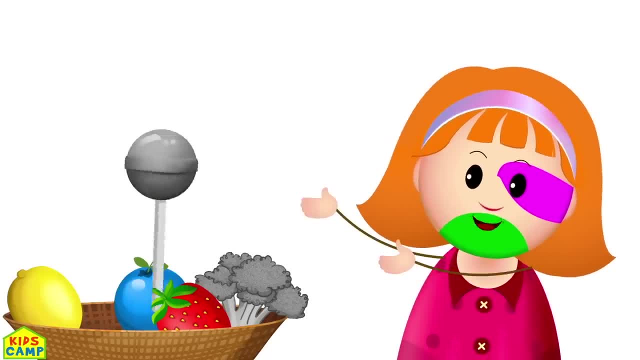 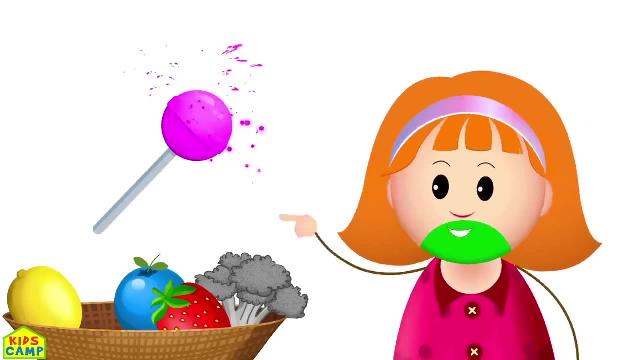 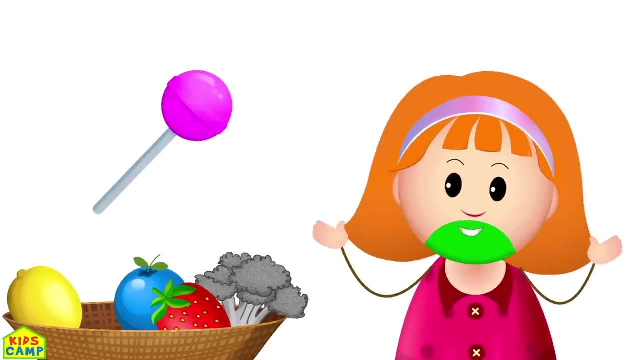 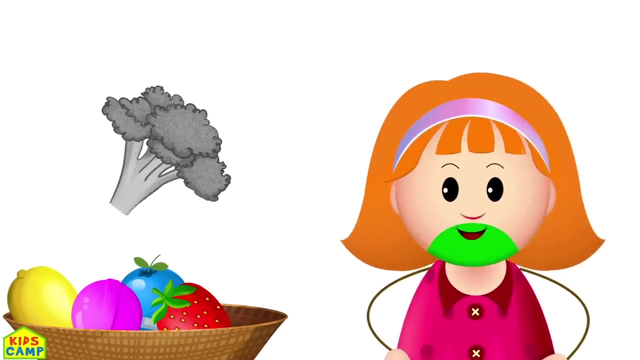 So sing out loud. What color is the lollipop? What color is the lollipop? Pink, pink. The lollipop is pink, Like a candy, Like an ice cream. This is wonderful, Just like a dream. What color is the broccoli? What color is the broccoli? Green, green. The broccoli is green Like a leaf And the trees. 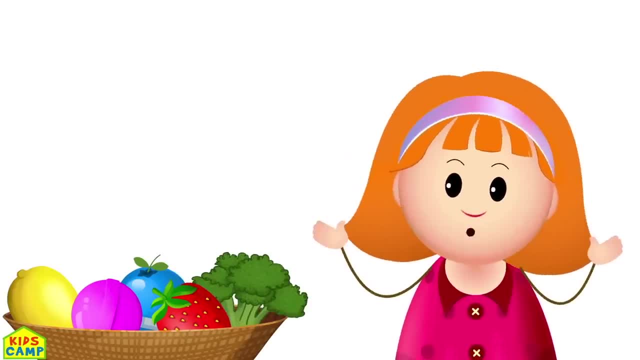 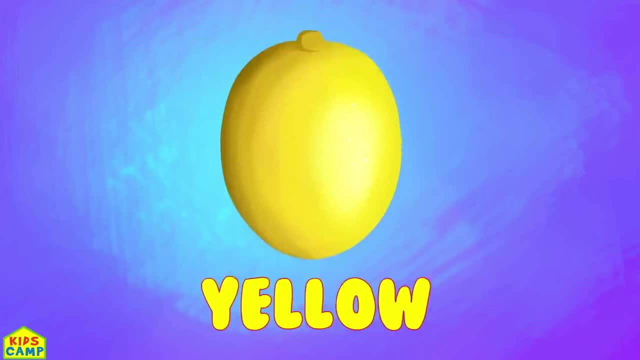 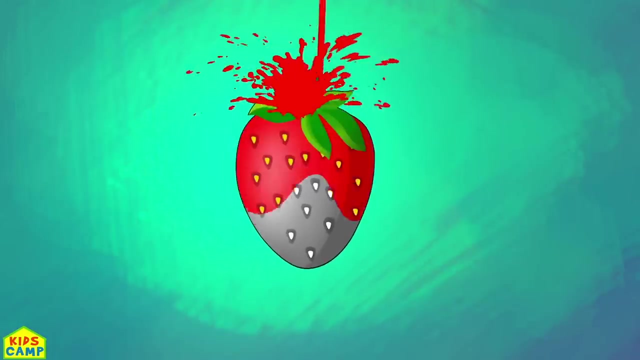 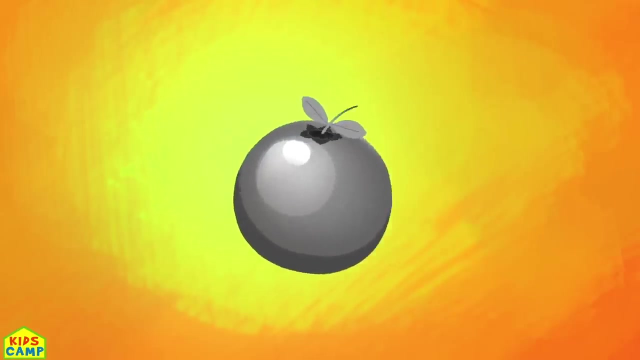 One more time, Sing along with me. What color is the lemon? What color is the lemon? Yellow, yellow, The lemon is yellow. What color is the strawberry? What color is the strawberry? Red, red, The strawberry is red. What color is the blueberry? What color is the blueberry? 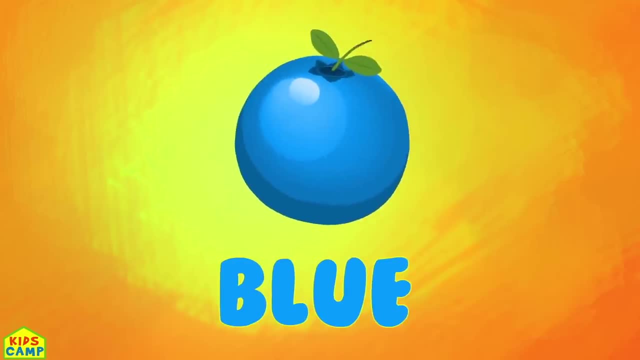 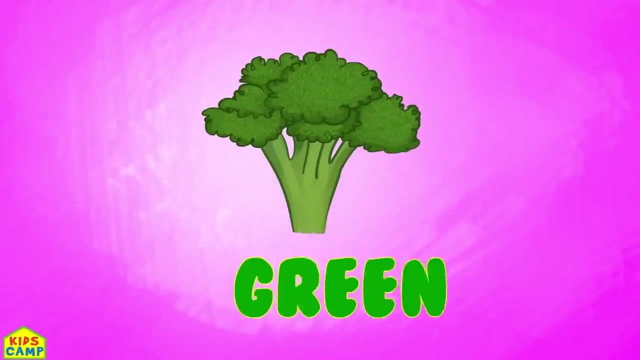 Blue, blue: The blueberry is blue. What color is the lollipop? What color is the lollipop? Pink, pink, The lollipop is pink. What color is the broccoli? What color is the broccoli? Green, green, The broccoli is green. 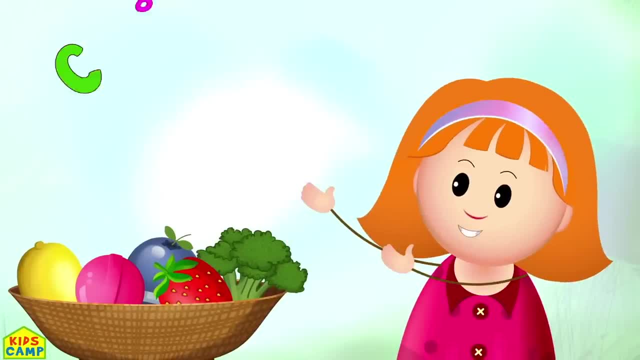 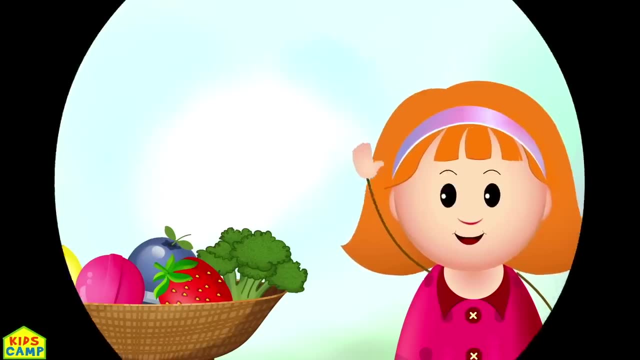 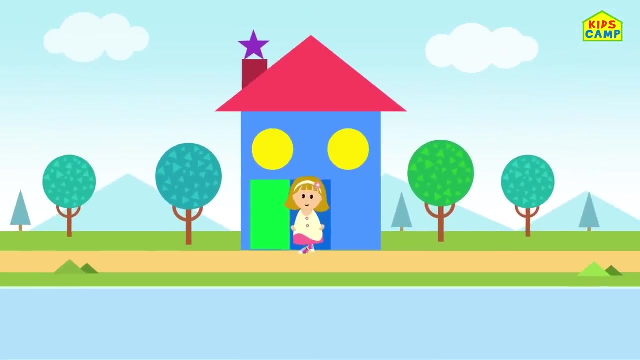 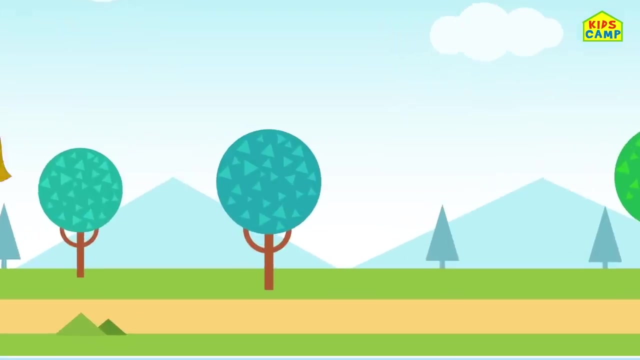 This was so much fun learning colors. Hope you liked it too. Bye, bye. Come on, Ellie, And this is my house of shapes Circle, Rectangle Star Triangle Square. As I was walking down the street, Down the street, Down the street, Mr Sun, I happened to meet. 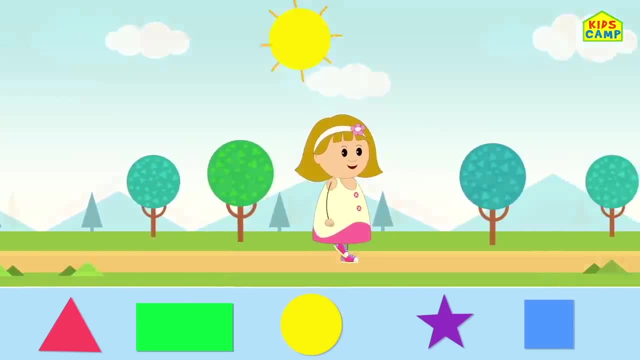 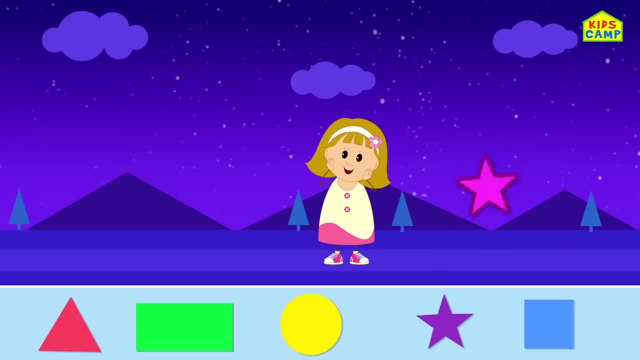 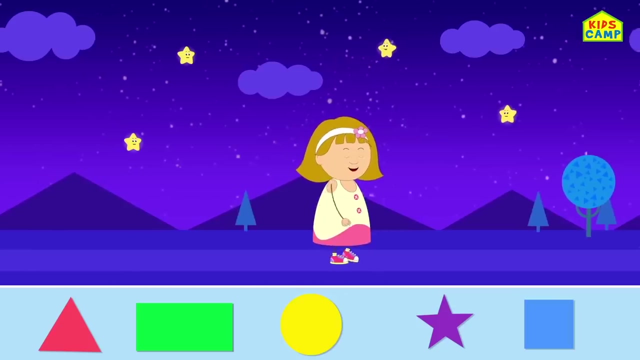 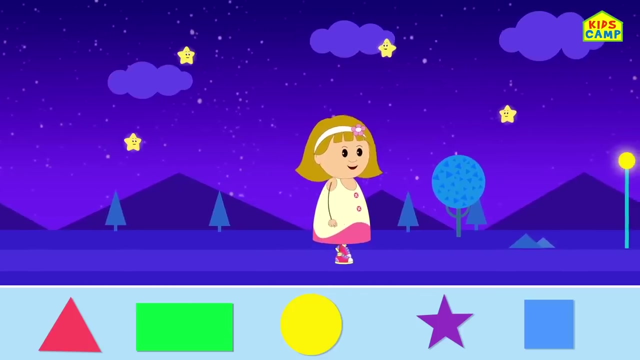 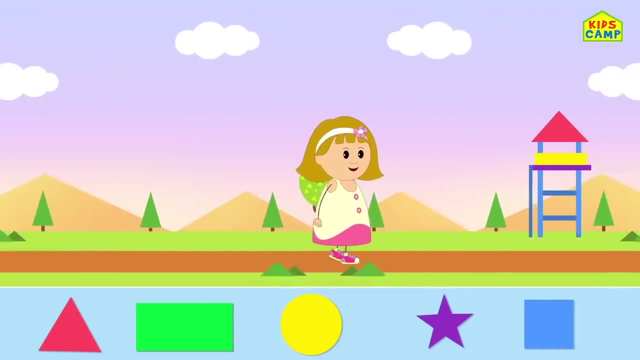 Hi there, Hi there, Hello Wow. Twinkle, twinkle little star. How I wonder what you are. Twinkle, twinkle little star, How I wonder what you are. Twinkle, twinkle little star, How I wonder what you are. 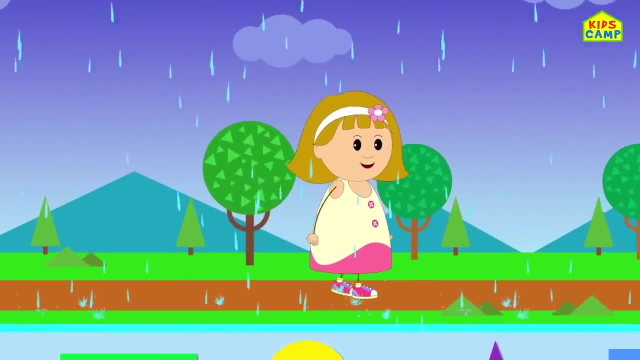 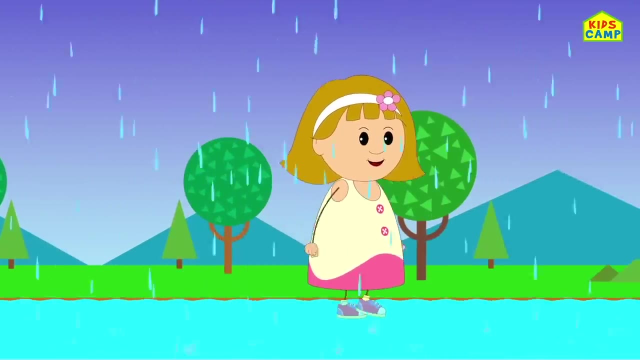 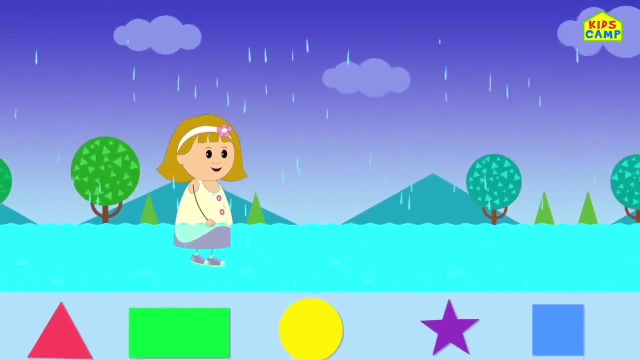 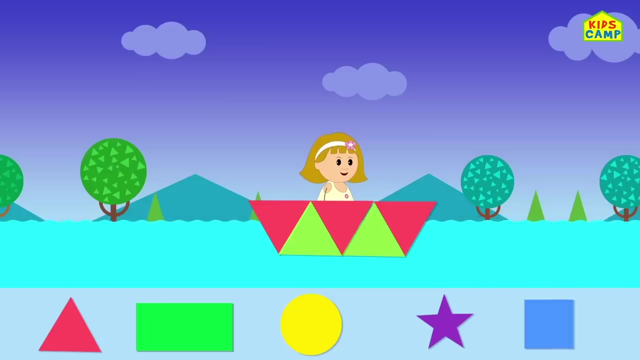 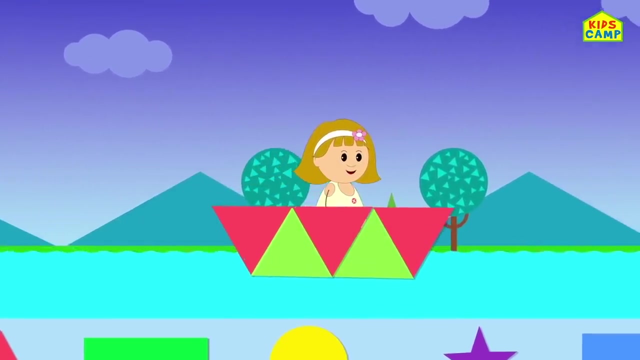 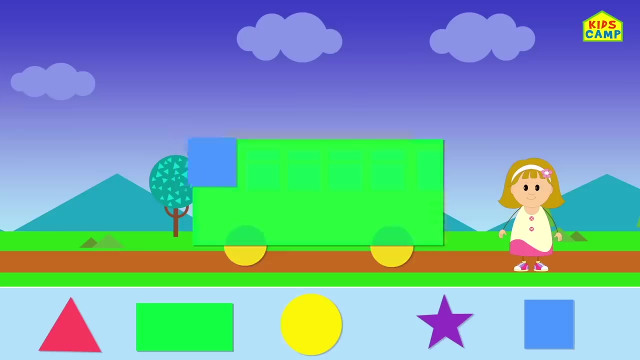 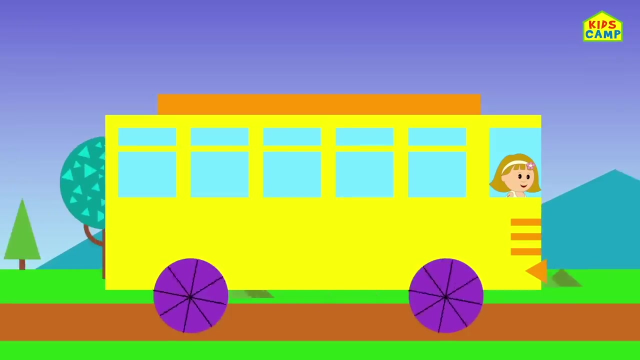 Wow, Ring ring. go away. Come again another day. Ellie wants to play Ring ring. go away, Let's play Ringing Ringing. Row, row, row your boat Gently down this stream, Merrily, merrily, merrily, merrily. Life is but a dream. 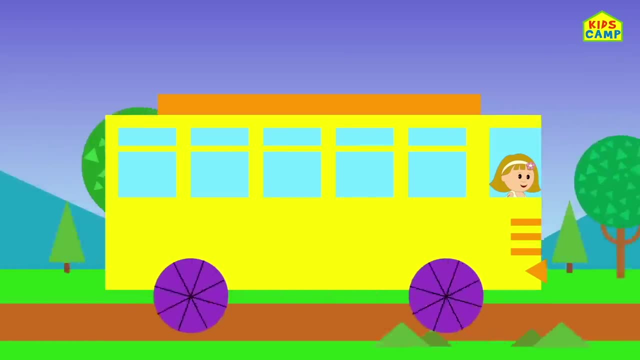 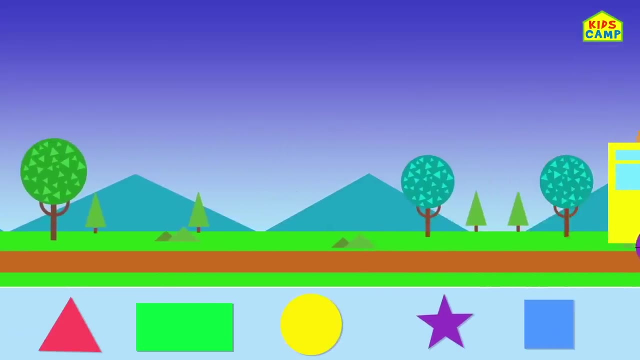 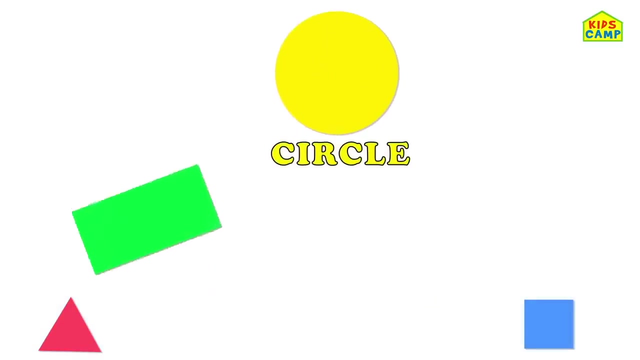 Wheels in the bus go round and round, Round and round, round and round. Wheels in the bus go round and round All day long Circle goes round and round, Round and round, round and round. Rectangle. it has four sides, Opposites but the same. 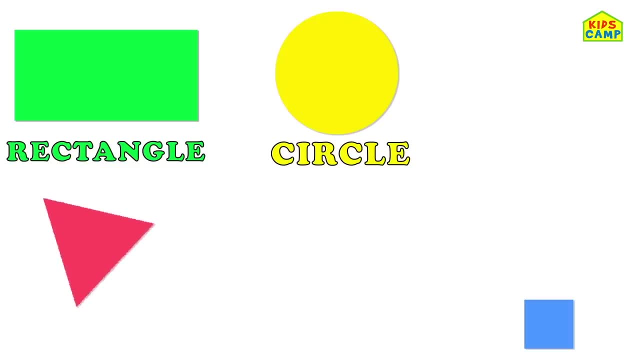 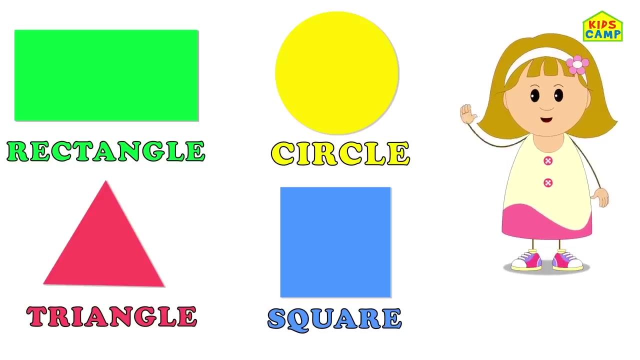 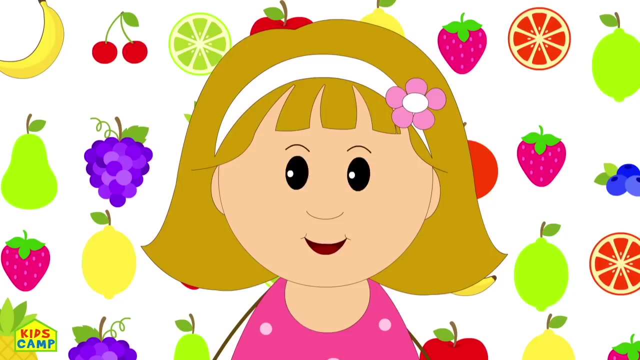 Triangle has three sides- Equal sides, with three sides. Square has four equal sides. All the sides are same. Yay, I love the shapes. Hope you love them too. This was super fun. Bye-bye, Hi, I'm Ellie. Let's have some fruity fun. 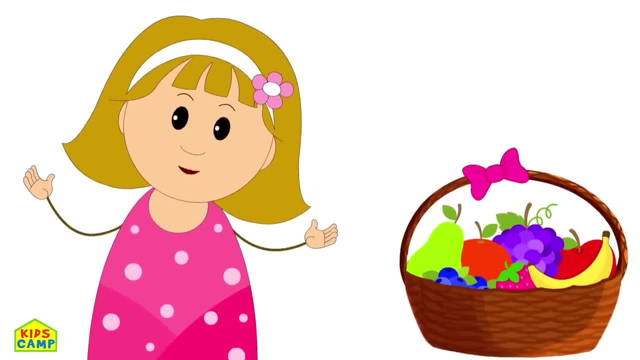 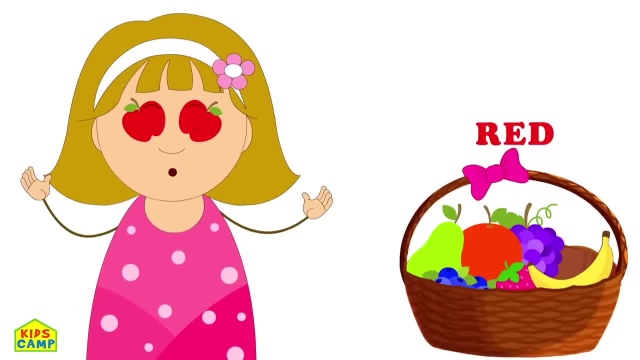 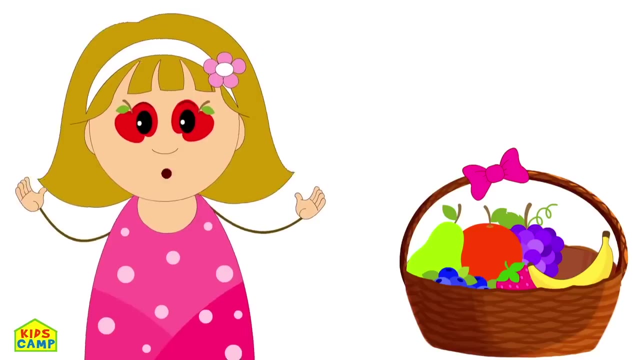 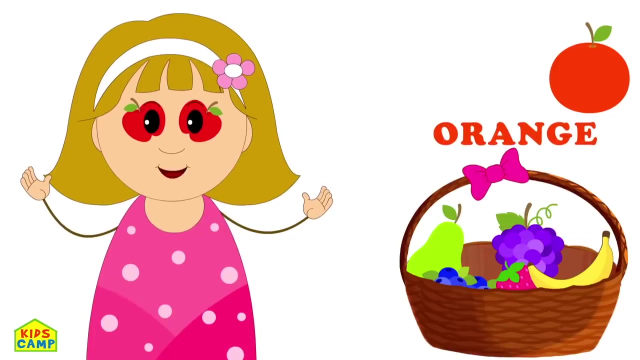 Here we go. Red color, red color- where are you? Red Apple of my eye, Orange color, orange color- where are you? Orange Slices in my hair, So tangy Pink color, pink color- where are you? 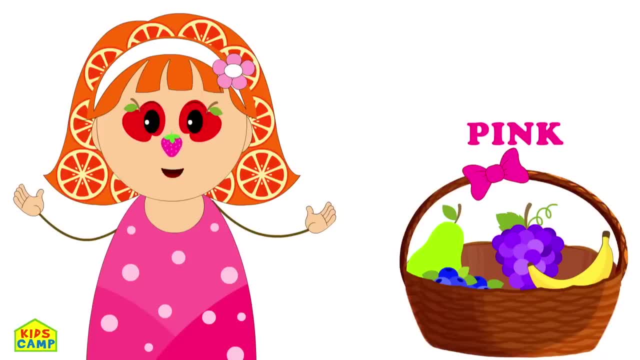 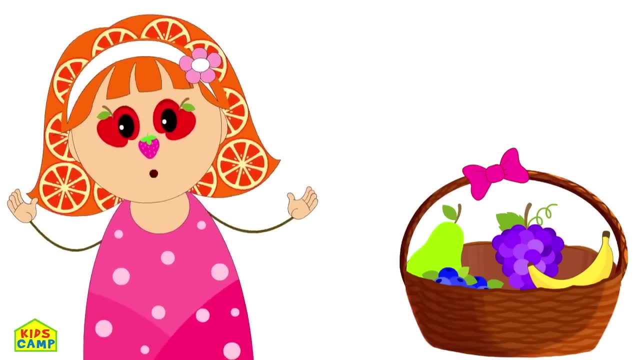 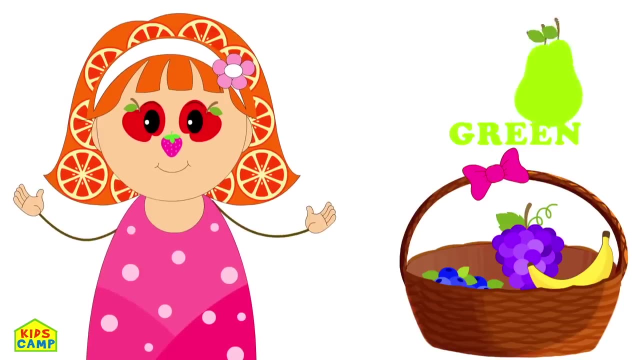 Pink Strawberry smells so good, Yummy. Green color, green color. where are you? Green Pears in my ears. Purple color, purple color. where are you? Purple, Ooh grapes. Blue color, blue color. where are you? 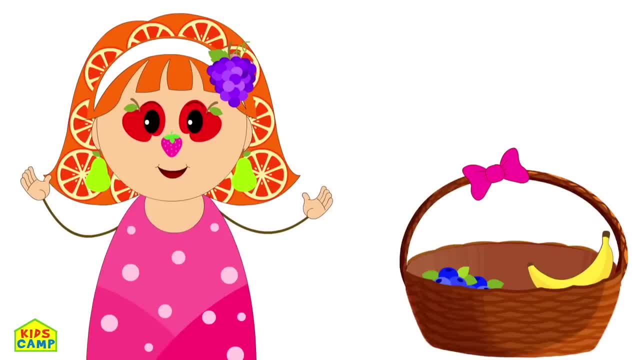 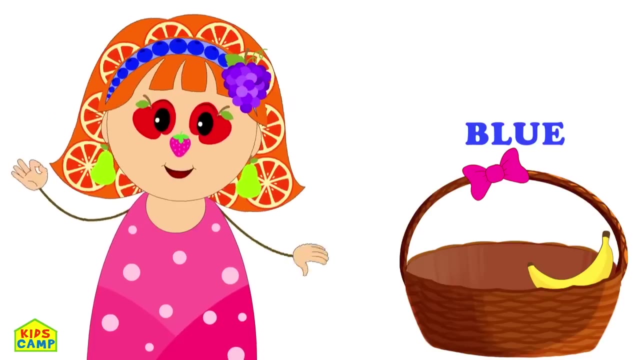 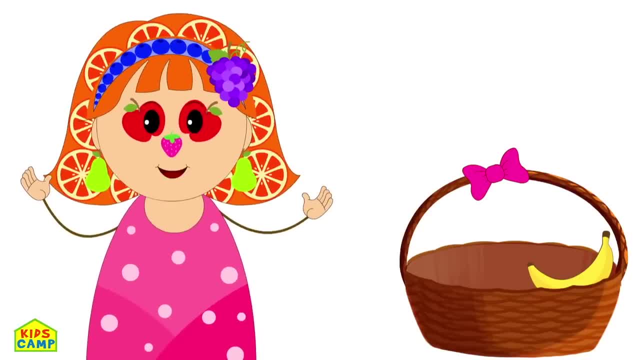 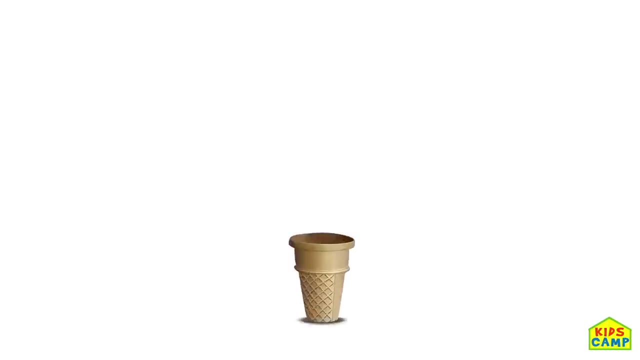 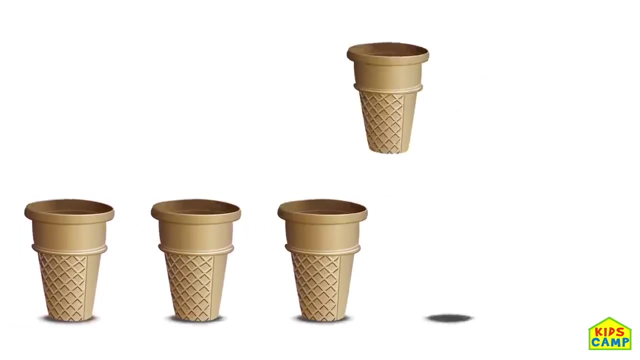 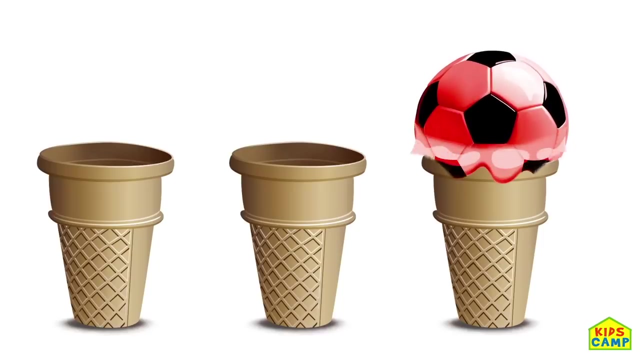 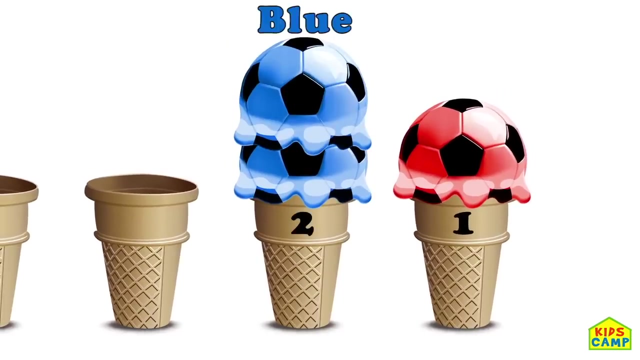 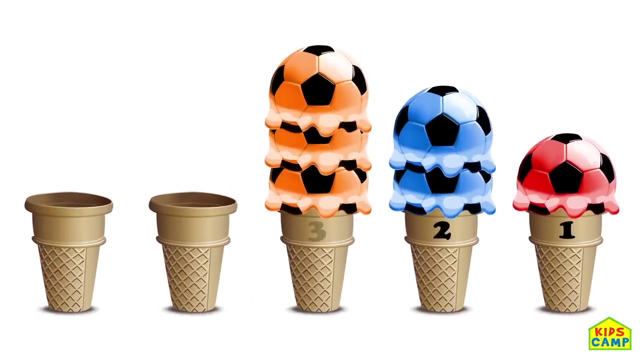 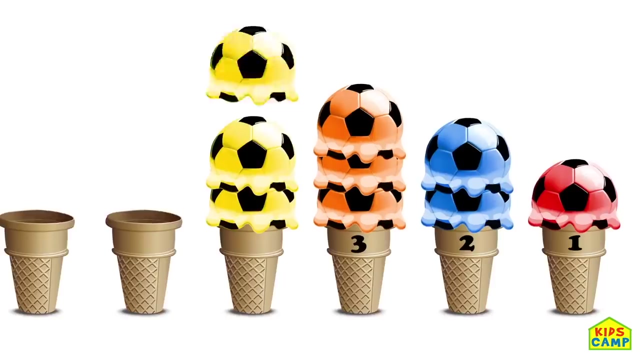 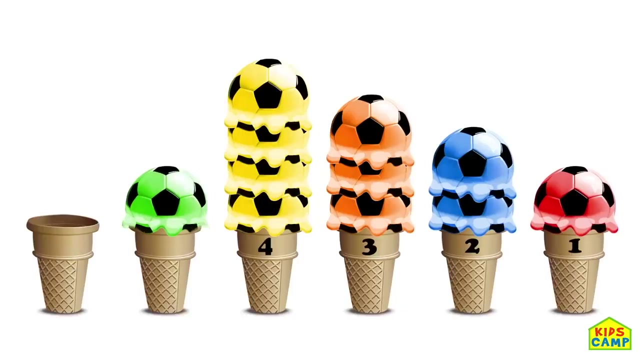 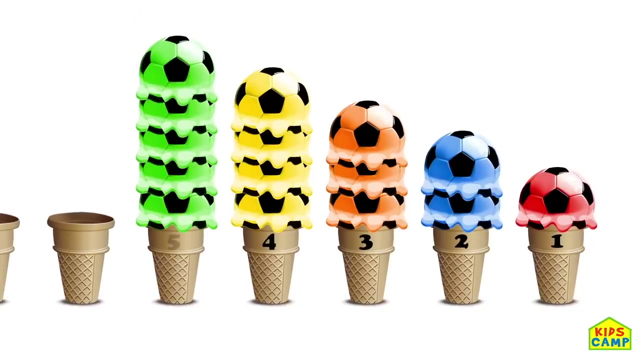 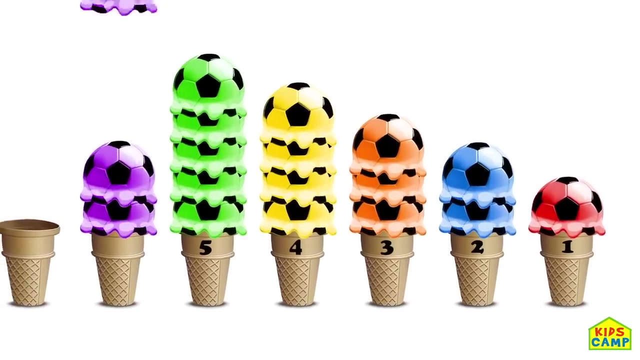 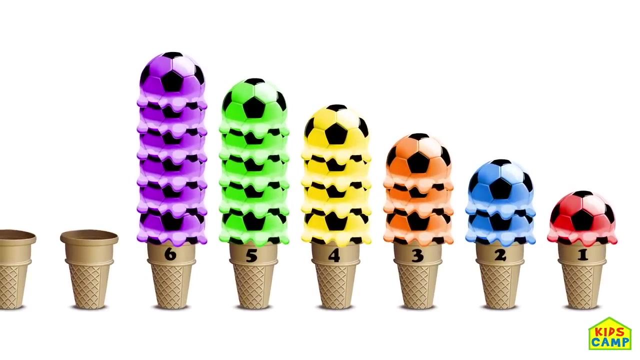 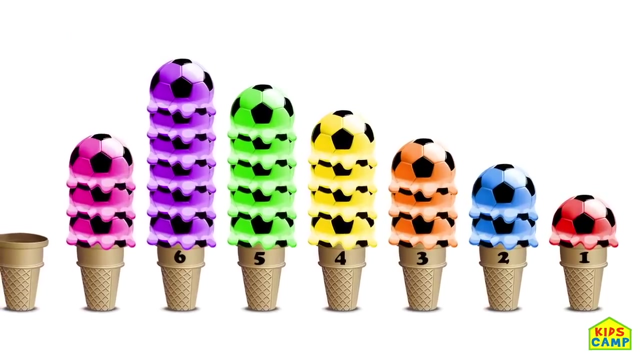 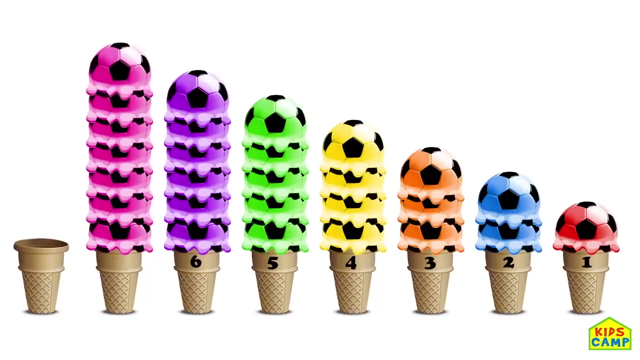 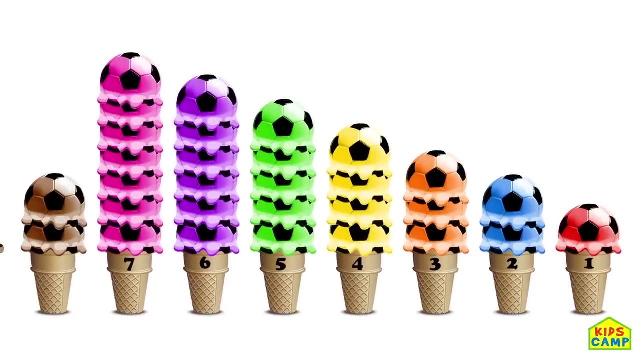 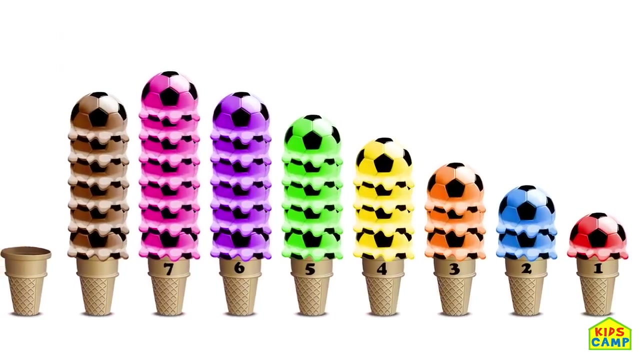 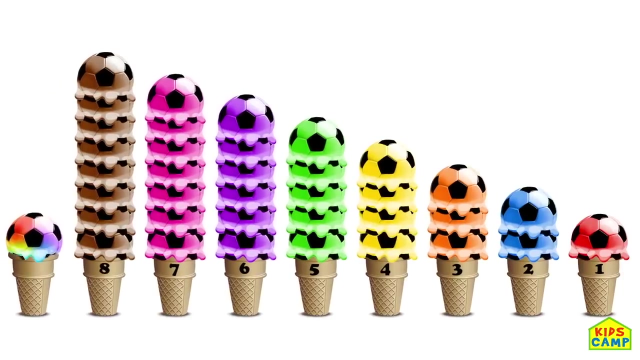 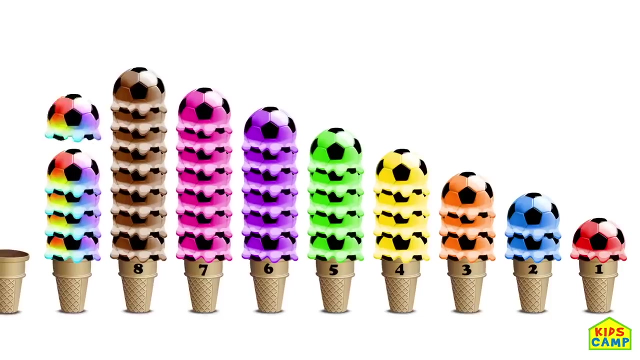 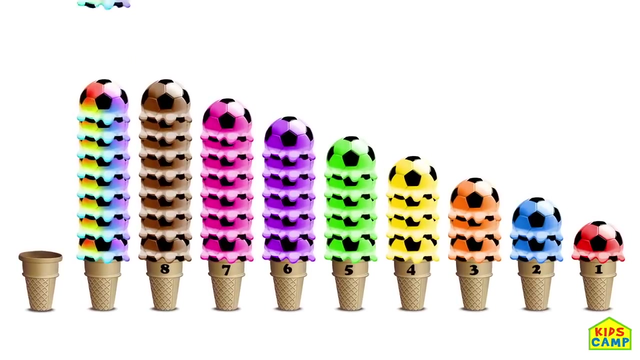 Blue, The yellow color. where are you? Yellow? This is my banana smile. This was so much fun. Red, Blue, Orange, Yellow, Green, Green, Purple, Pink, Brown, Yellow, Rainbow, Blue, Yellow, White.